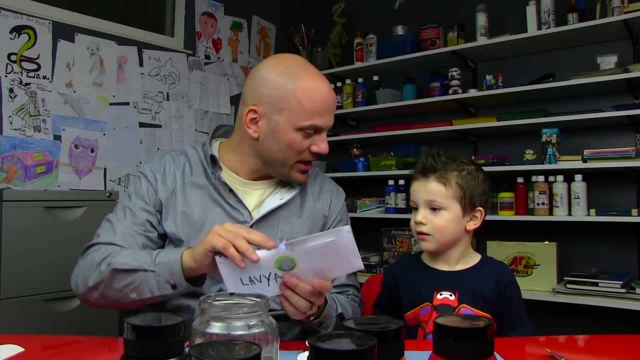 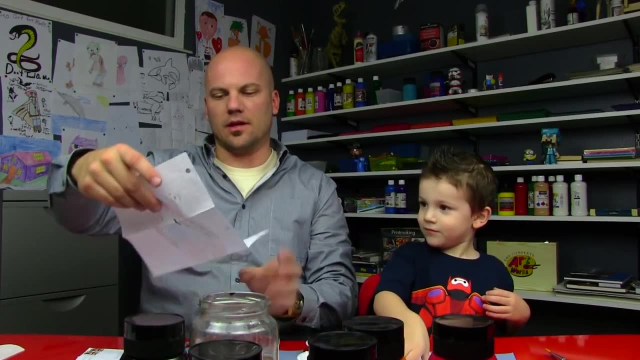 This next one's from Laya Patel and she's from Florida. Isn't that cool, Yeah, Alright. oh, she's got a lot of drawings. You wanna open that one And I'll open this one. Oh, it looks like a cupcake, Yeah. 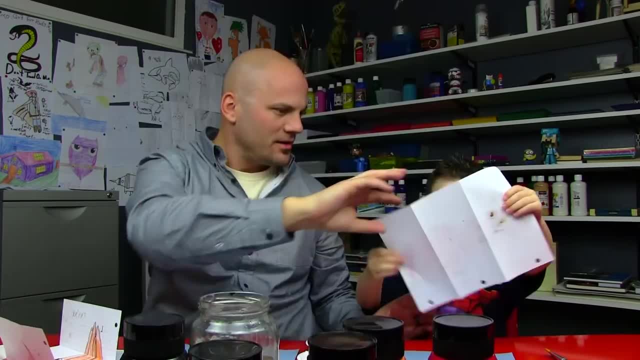 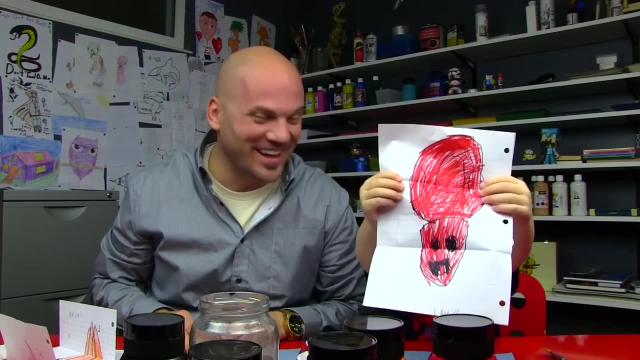 That's an awesome colorful cupcake. Hold it up like this. Here you go like that. Good job, You're holding it, Good job, That's a really cool mushroom. huh Yeah, Yeah, you're being a good helper. 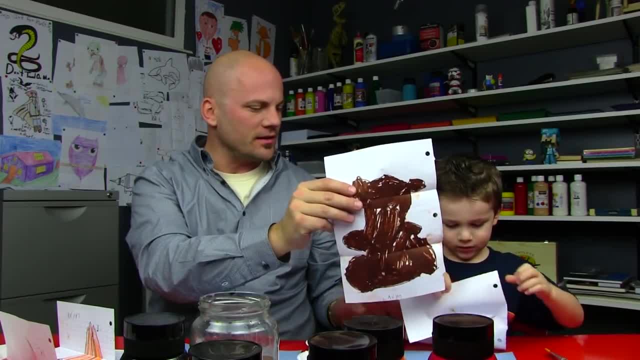 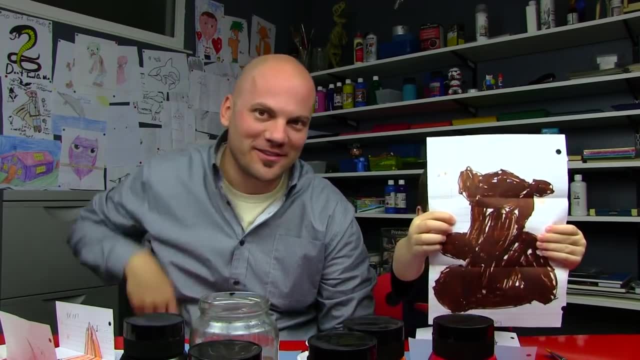 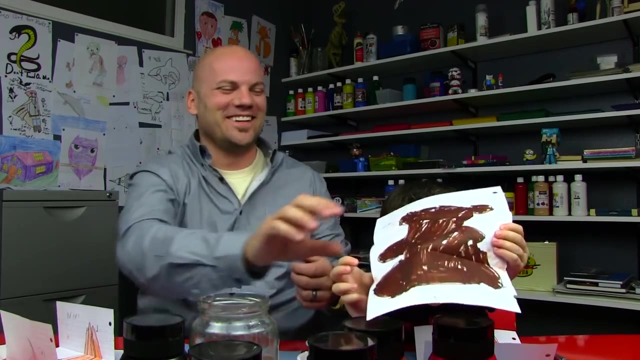 You wanna hold the bear up? Hold the bear up so that all our art friends can see Here. You can't quite get it close to the camera, can you A little closer, Closer? Good job, Austin. That is really cool. We love that little teddy bear, huh. 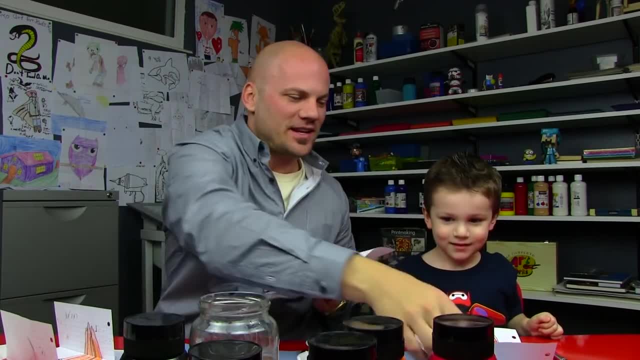 Yeah, Awesome teddy bear. Thank you so much, you guys, for sending this in. Alright, should we paint our snowman? Yeah, Okay, let's do it. So we got all of our paints and we got our supplies. 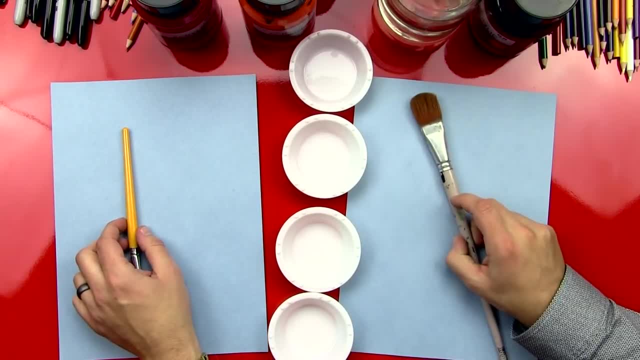 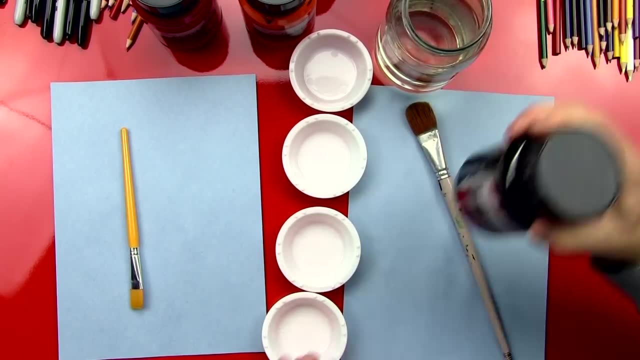 We got paper, Yeah. We got our paint trays, Yeah, And we got our paint brushes, Yeah, Right, Yeah. And we got some water, Yeah, And our paint, Yeah. Alright, we're gonna, yeah, yeah. 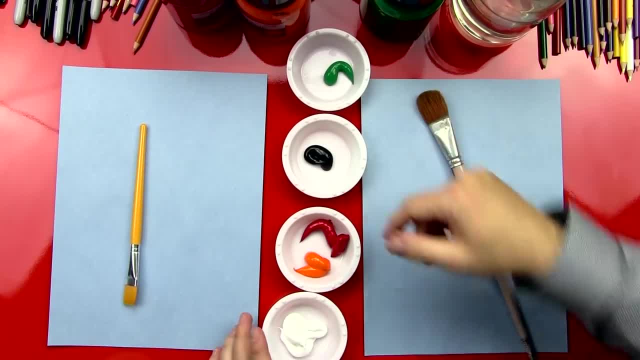 We're gonna put all of our paint in our paint trays and then we'll keep going: Okay, Okay, that's all, Yeah, Okay, we got all of our paint in our trays. huh, Yeah, And we got our paint. 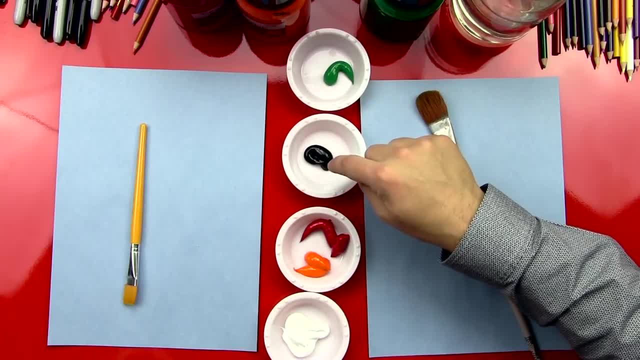 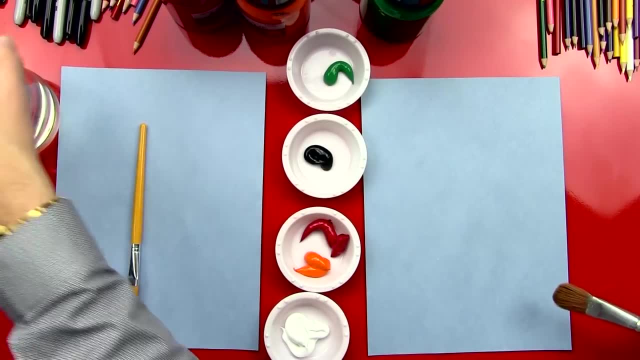 Yeah, And we got our paint. Yeah, White, White, White, Orange, Orange, Red, Black, Green, Green. Yes, And we're gonna use all these colors. And we got our water. I'm gonna put this water next to you. 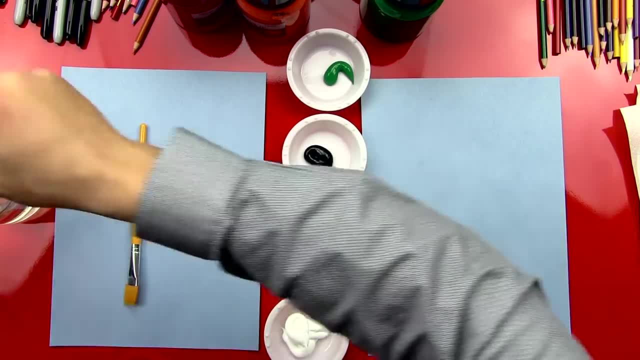 And then I can. it'll be close to you and I can reach over you. Yeah, Then we also have paper towels. Yeah, So we can dry off our paint brushes. Yeah, Okay, First step, Let's get our paint brush a little wet, alright. 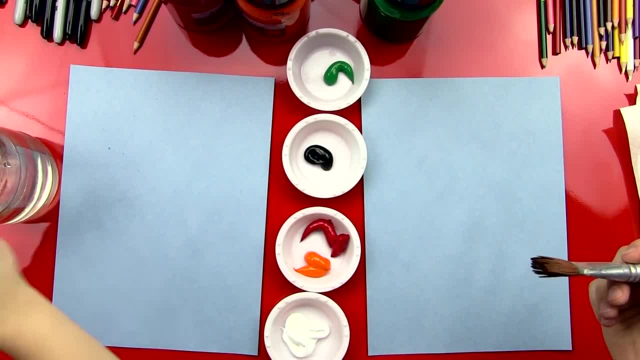 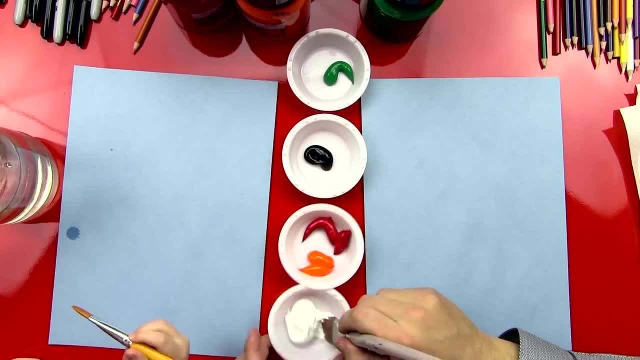 And we are using acrylic paint, but you can really use any paint for this. Yeah, You can use watercolor if you want. Yeah, watercolor might be a little difficult with the white, but if you have acrylic or tempera it'll work really well. okay, so we're gonna get a lot of white on our 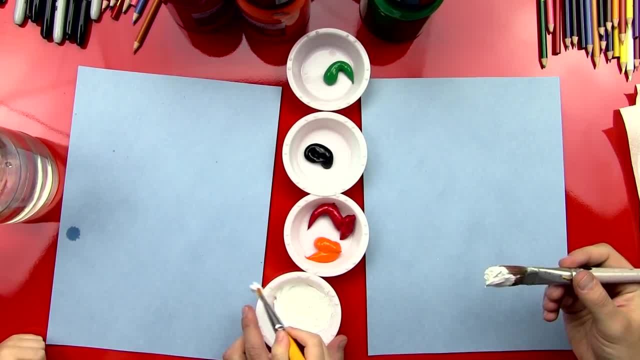 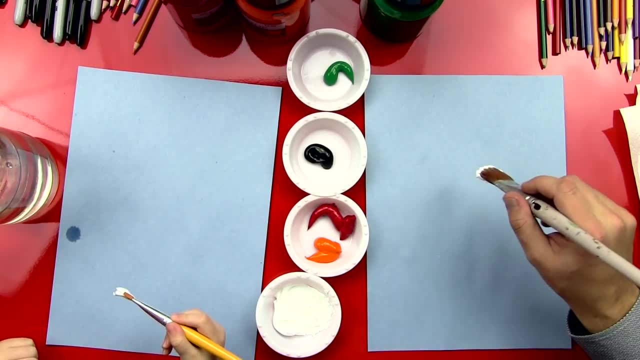 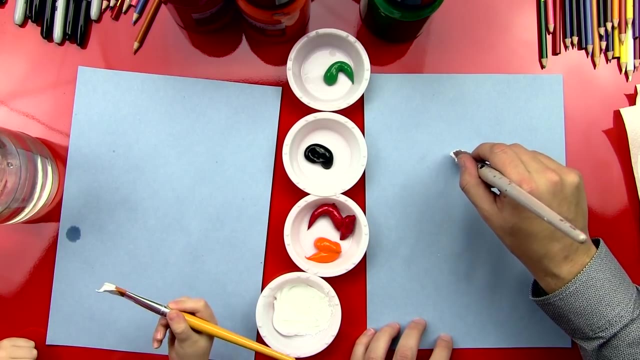 paintbrush. okay, there you go, bubby, all right, and I got some water on your, on your paper, all right, first we're gonna do a bird, a big giant circle, in the middle of our paper. okay, watch me. and then you do yours. all right, so we could. 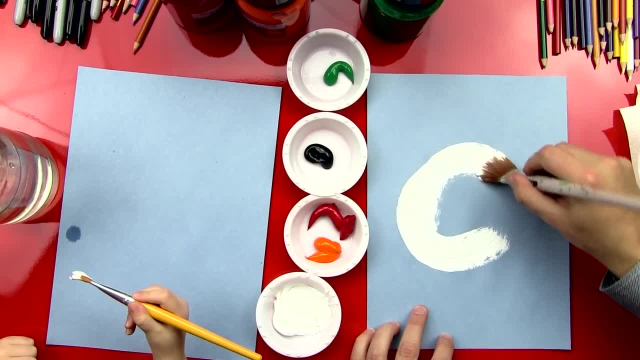 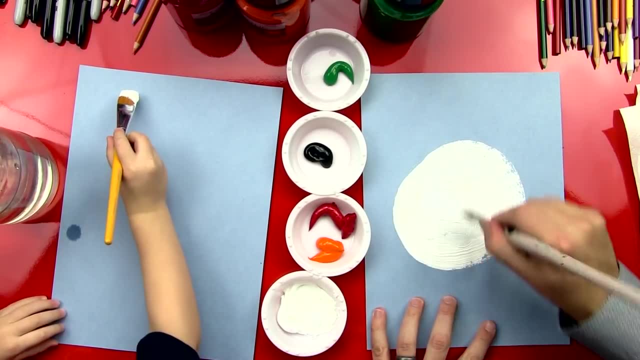 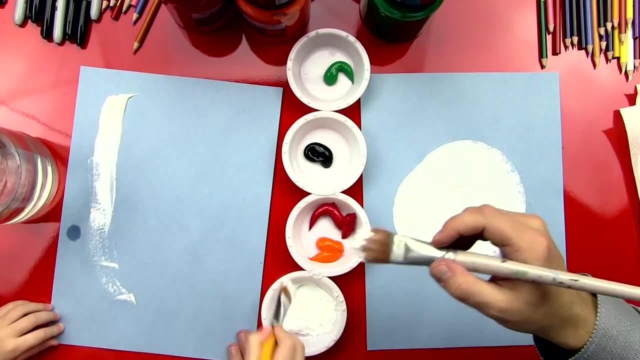 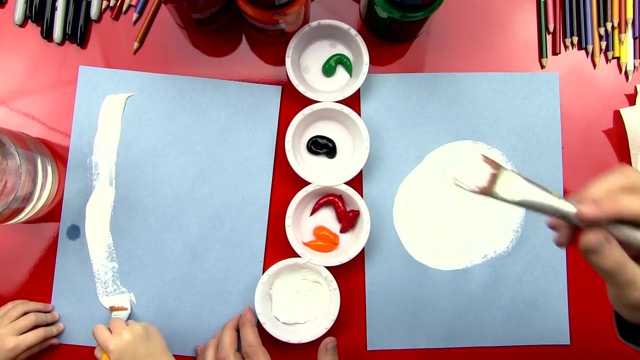 go like this: we're gonna do a big giant circle right in the middle of our paper. okay, you do yours. okay, right here, do a big circle right here in the middle. yes, you do, you know we might need a switch, yeah, okay, let me help you for one second. 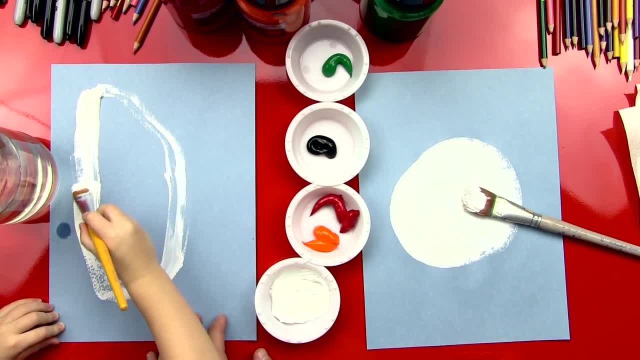 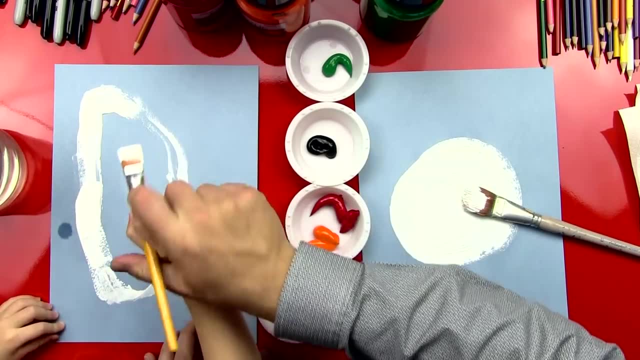 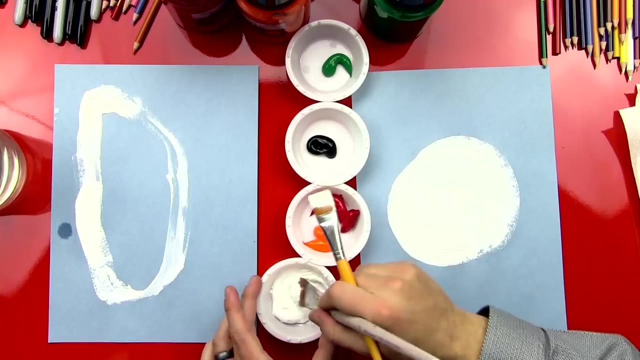 oh, you can do it, you did it just right. okay, look, you got a lot of paint up here in the corner and if you mix it, see if you bring it out here here let's switch. you try this paintbrush, see if this one works a little bit better. let me get some more water. one sec, get more. 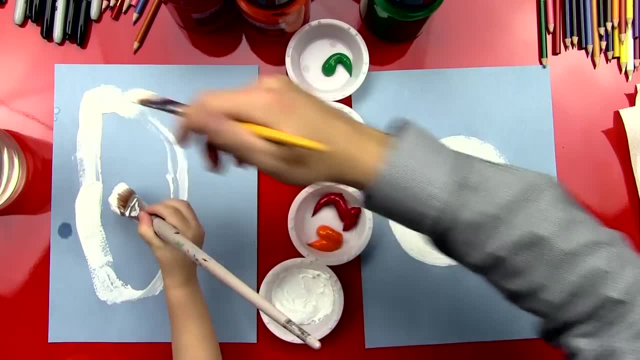 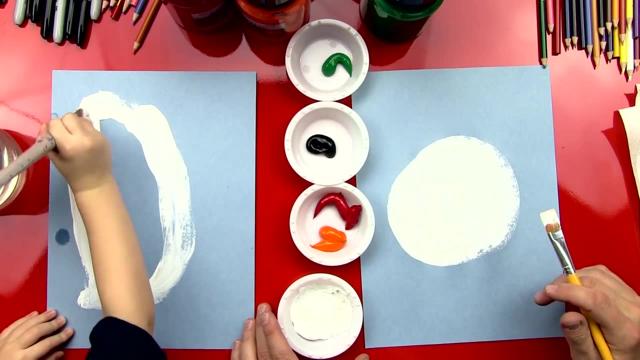 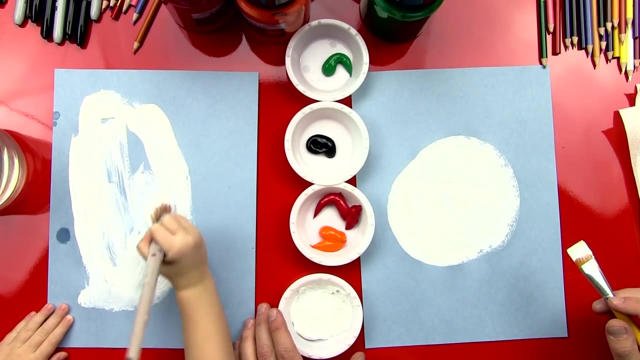 paint. okay, now you do it. see if you can paint in your big circle. yeah, that works better. huh, yes, and paint it in paint in the middle. perfect, awesome, keep going. you're doing such a good job. is this fun? yeah, yes, it is. I'm having fun with you and we just started. are you done? all right, so watch. 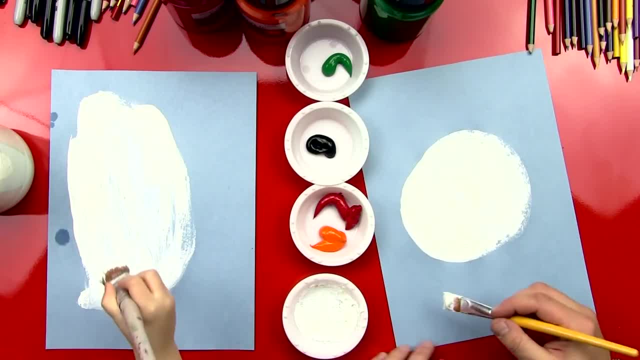 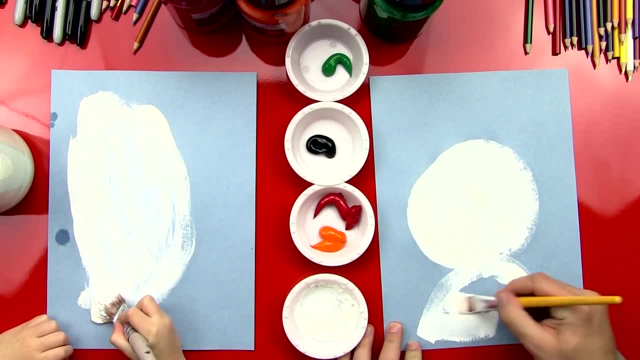 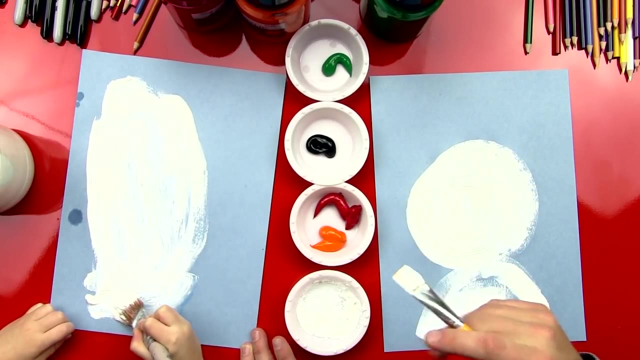 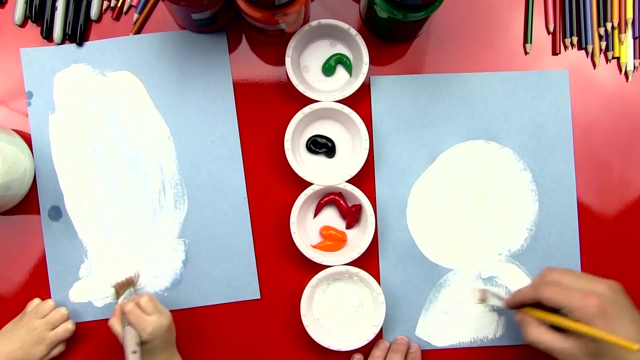 me, I'm gonna get more white on my paintbrush and we're gonna come down here and we're gonna do a big you upside down you and then painted it. can you do that? so do a big you, yes, good job- and then paint it in doing awesome, Austin, and we're gonna paint. so 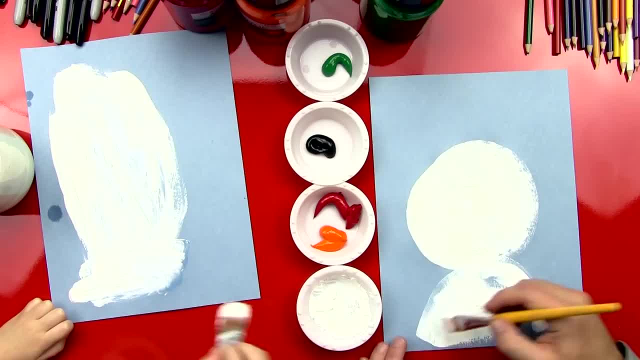 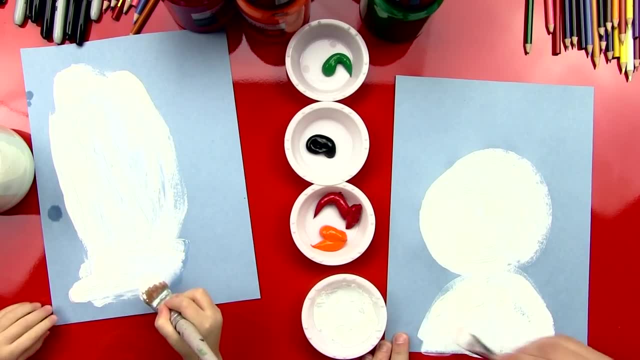 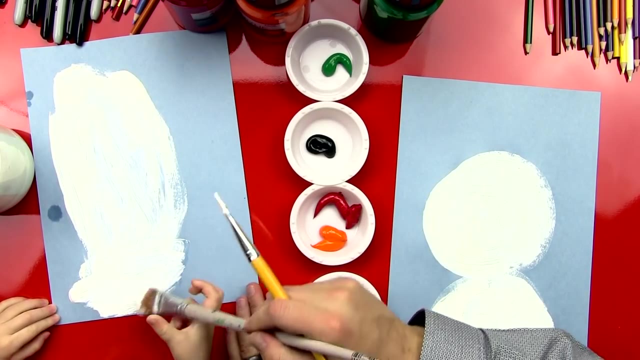 if our art friends at home, you guys probably want to put some scratch paper underneath your painting and then you can do all the way up to the edge. we're just gonna- I'm just gonna- pay on the table, so be sure to ask your parents at home if it's okay to paint the table, because it's probably not all right, good. 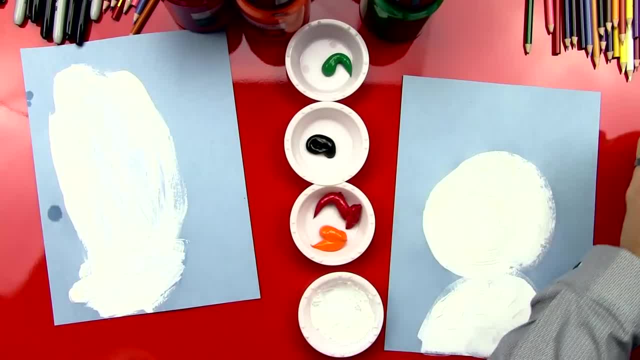 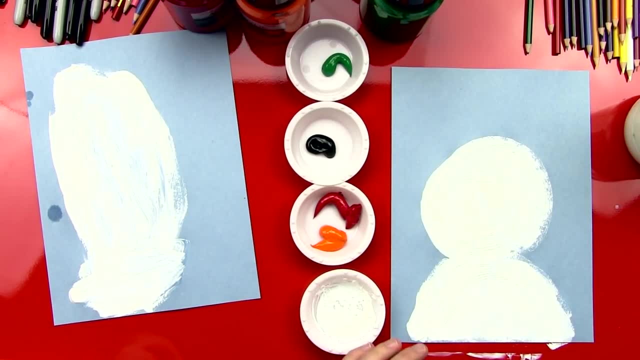 job, Austin. hey, now we're gonna rinse it off. okay, now we should do. should we do the ice? let's get a little black and we're gonna do a smaller paintbrush for this, so we have a smaller one. you can use this one, Austin. all right, so we're gonna get a little black on our paintbrush, you do. 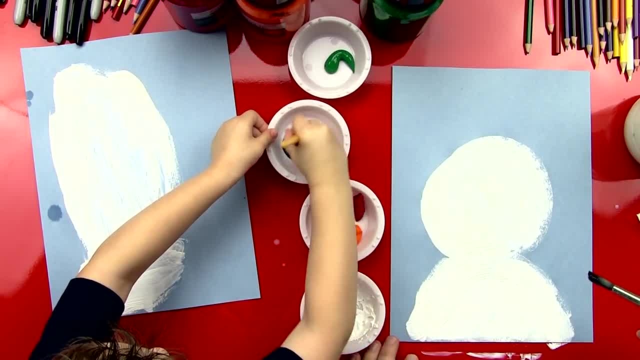 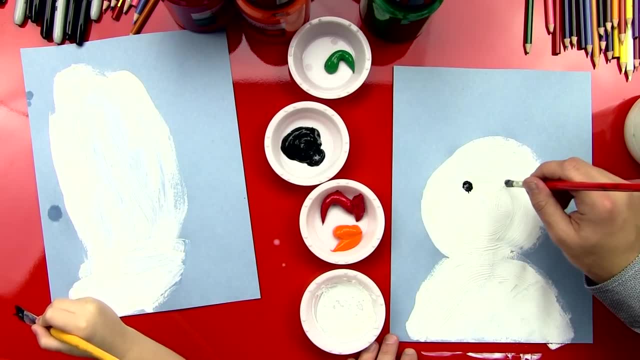 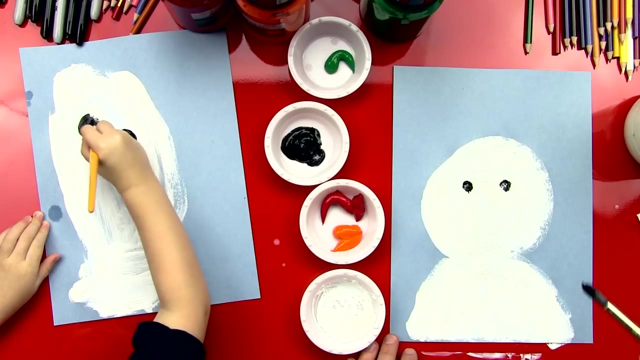 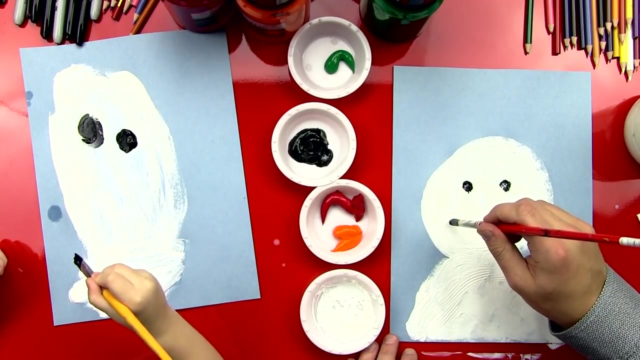 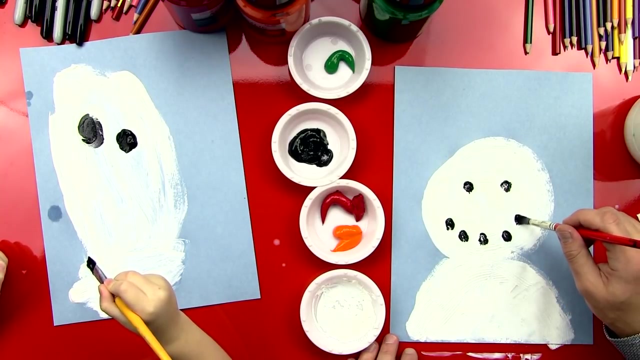 that. get some on there. good job, awesome. okay, we're gonna do two eyes, so we're gonna do two little dots. watch this. one, two, one, two. good, okay, now let's do the mouse, so we're gonna get a little more black. okay, watch this and then you do yours. you're gonna do dots, okay, one, two, three, four, five, do. 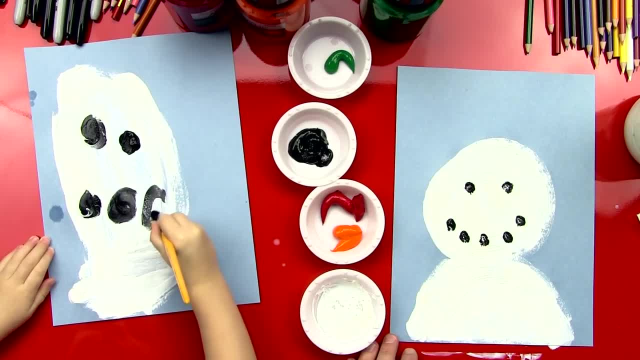 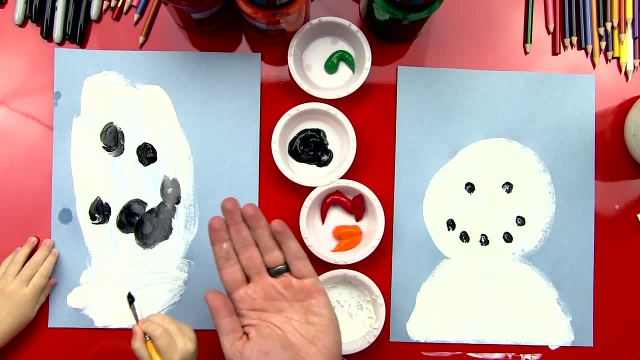 it in a smile. you can just do three dots. you wanna just do three? good job, give me five. dude, that's some awesome counting, all right, okay, now let's rinse off our paintbrush. okay, okay, austin, now we're gonna use. we're gonna use that first brush that you had, okay. 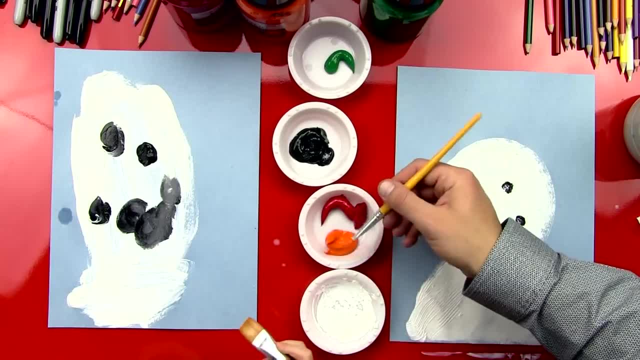 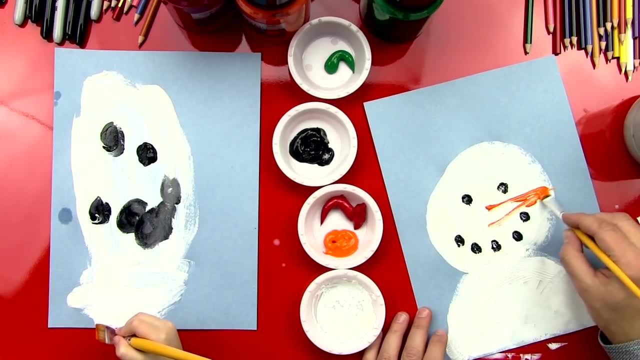 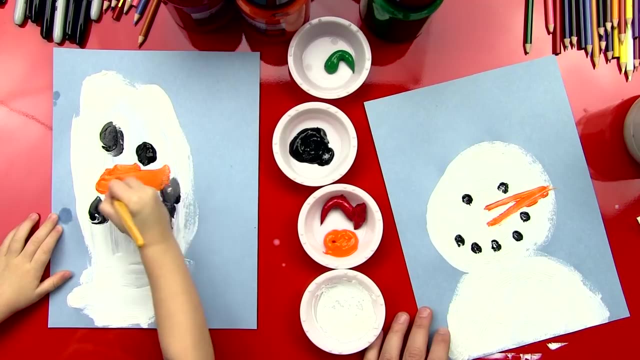 and we are gonna use orange for the nose. here we go, we're gonna do a v, so we're gonna go like this out and then back in like that. yes, a v, yes, that is perfect, perfect. you even did all the coloring and i was gonna do that on the next step. 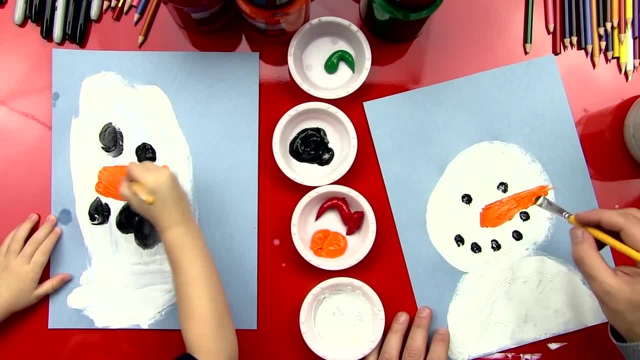 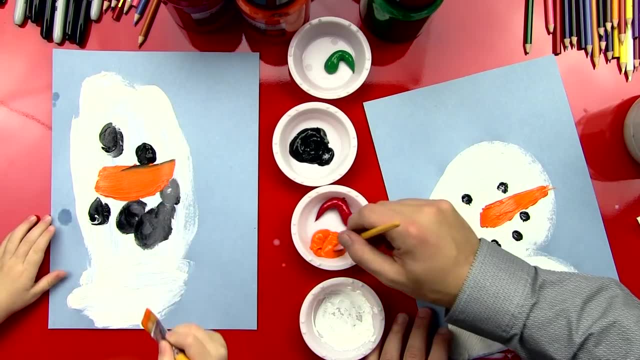 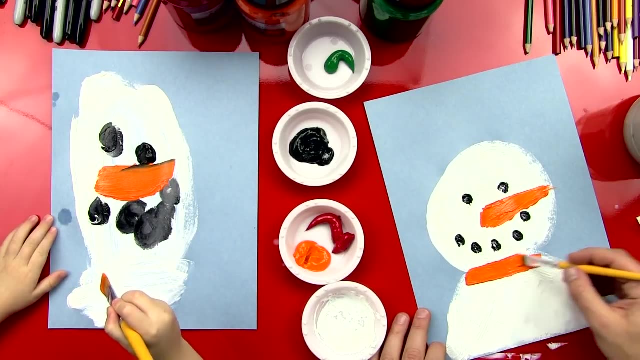 okay, you get some more. i like your carrot the best. your carrot is awesome. all right, should rinse it off. oh, actually, let's. let's do a little more orange and we're gonna do the his scarf. so we're gonna put a line right here for our snowman scarf. 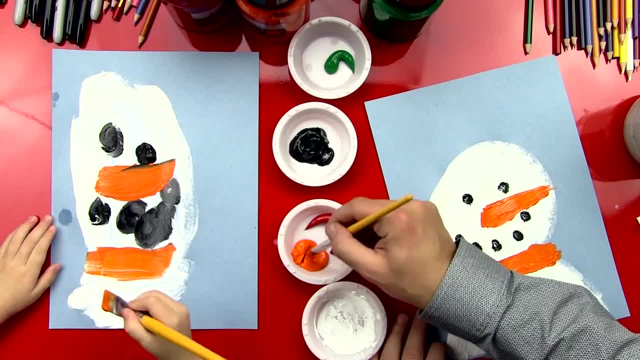 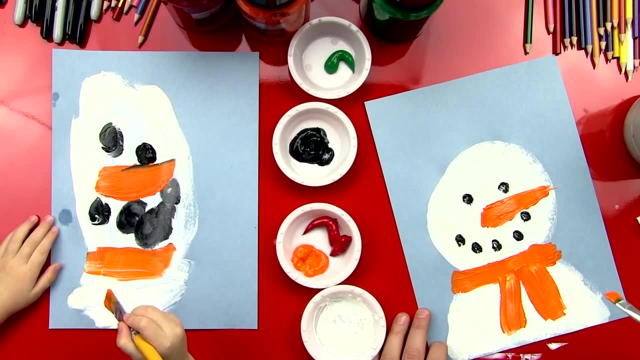 perfect, okay, and then we're gonna do two more down, one like this and then another one like this. okay, you do that, yep, and do another one. oh, that's so awesome. okay, let's rinse it off. okay, austin, this next part is gonna be a little trickier. watch me, we're gonna do red on our paint. 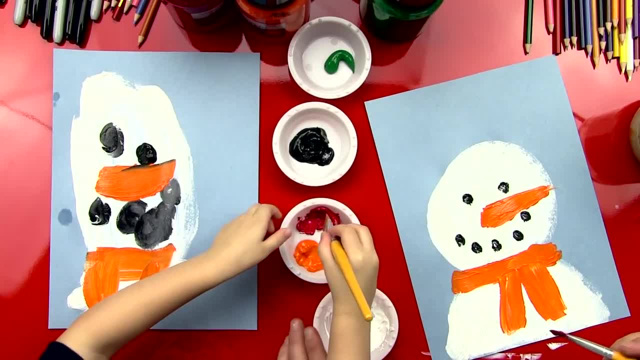 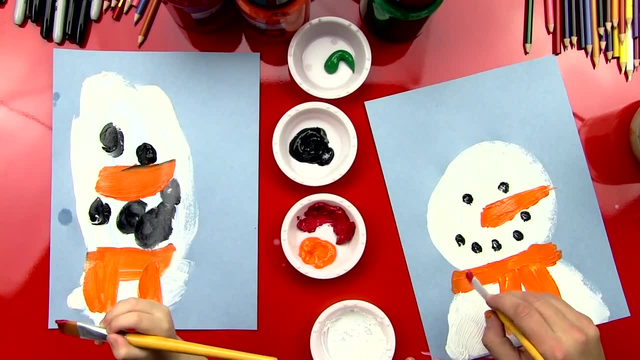 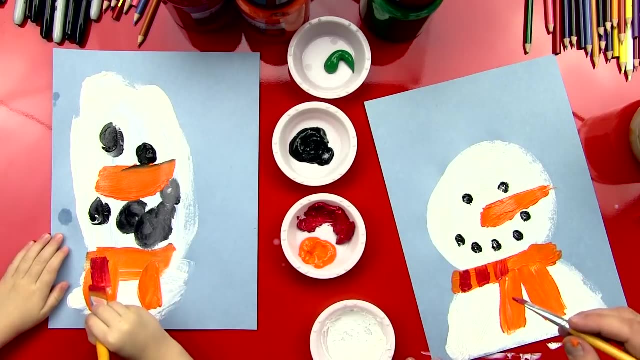 brush, okay, and then we're gonna put stripes on our scarf. okay, watch me, we're gonna be really careful when we do this part. here we go do little stripes, so we do little downs. one, two, three. can you do that? just little ones: one, two, three, four. good, little tiny ones. okay, now we're gonna. 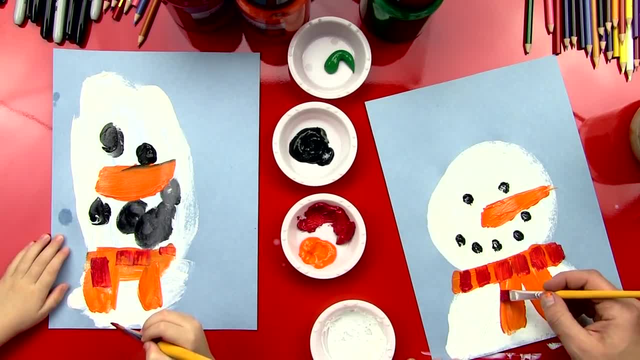 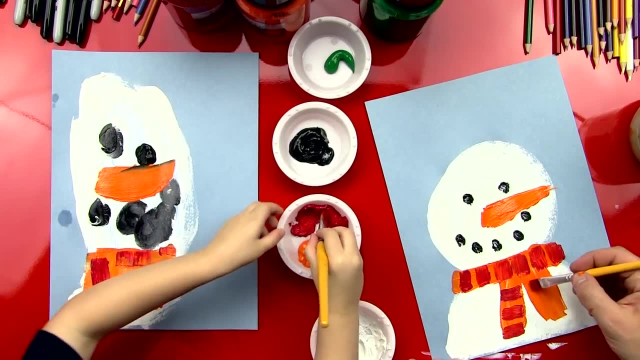 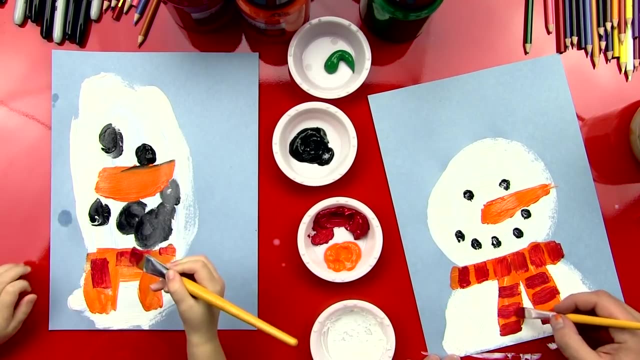 do stripes going down. i know maybe you could do do a couple stripes like this on the scarf going down. okay, a little more, little more. yeah, you can get as much as you want. you got a watch, you got a lot. yeah, perfect to do it. striking that way, yes, 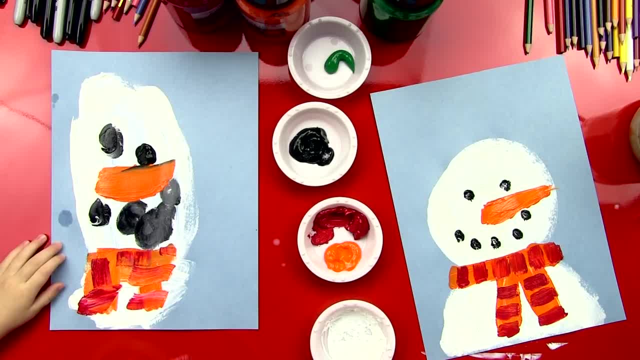 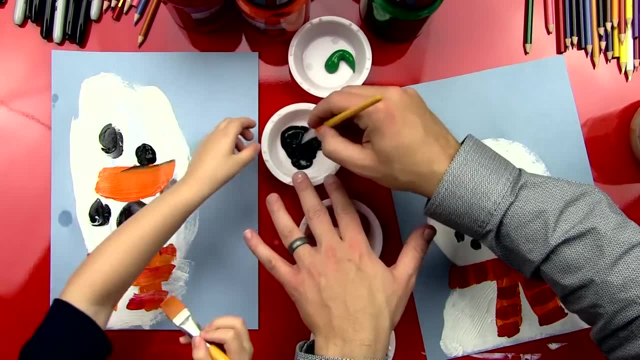 good job. okay, let's rinse it off again and we'll switch to black. okay, austin, now we're gonna get black. we're going back to black and get some on your paintbrush. we're going to do a swatch of tender dry Красить. 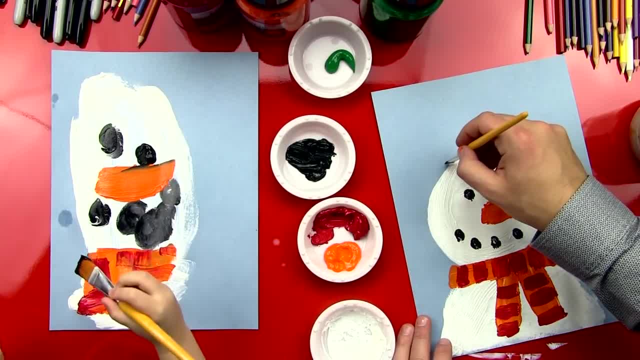 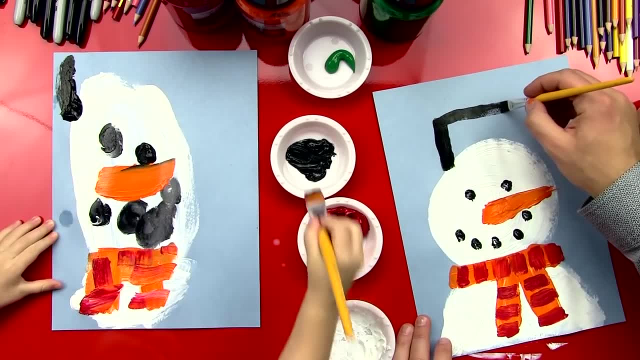 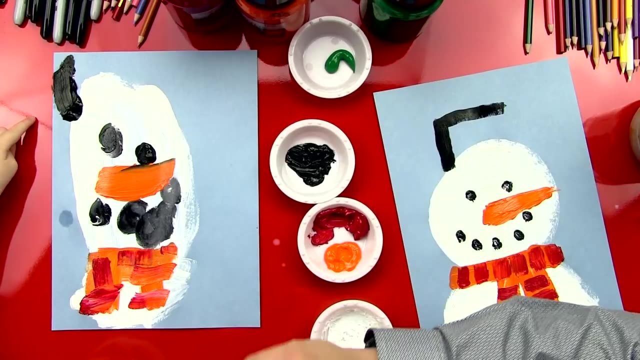 okay, let me well darken this side of the scarf a little bit. okay, square on top. okay, We're going to go up. Can you do that? Go up, Yep, And then over. Oh, I don't think you need more, You got a lot on there, And then we're going to go over, It's okay, You know. 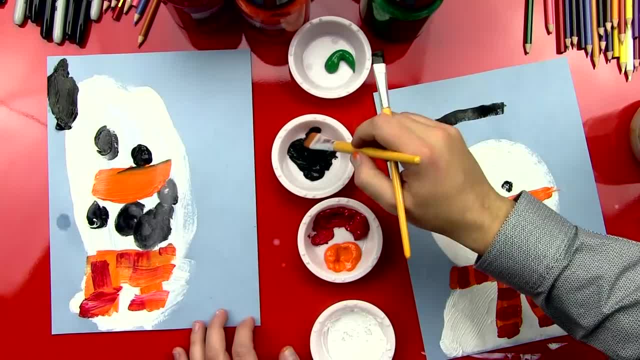 what You got, a ton on your painting right there, We'll get it. We'll move it over here and then you don't have as much and we'll scoot it down so you can reach it There. you go Ready. So now we 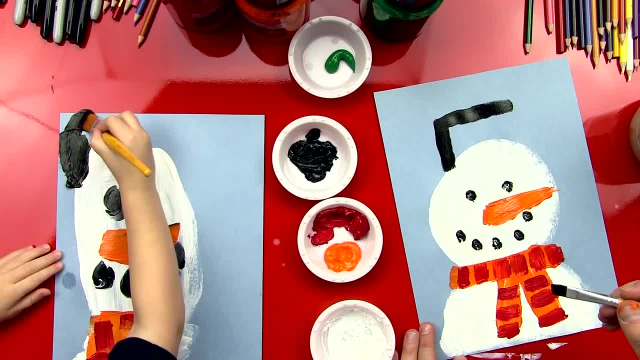 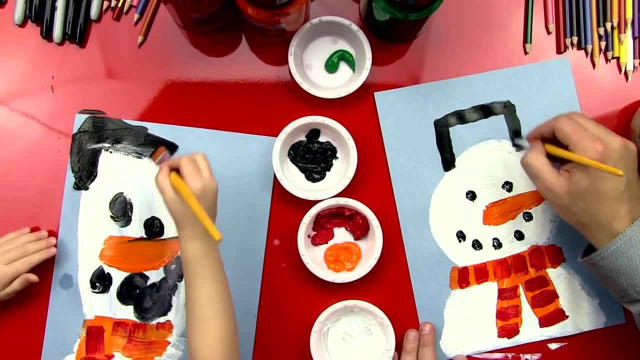 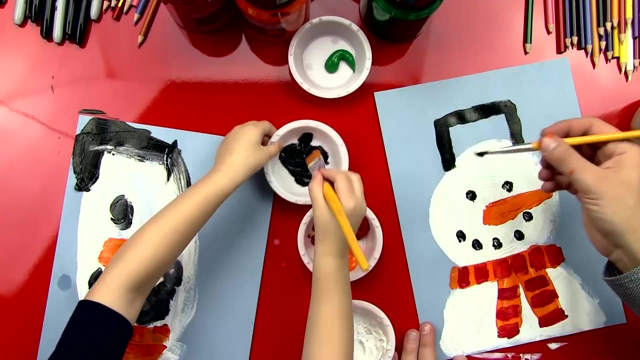 do the top, Do the top of your hat. Yes, Keep going a little further, Okay, And then we're going to go down. Okay, And then we're going to do a big line that goes across: Here we go. This is a lot. 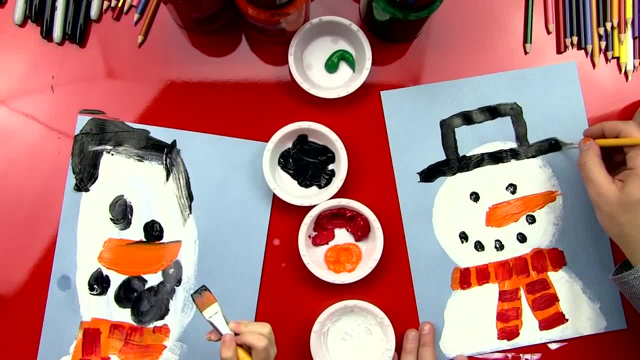 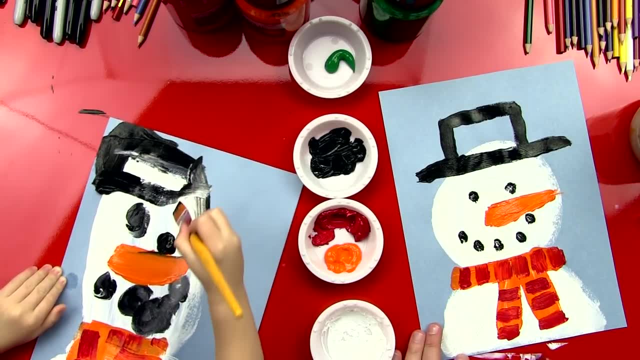 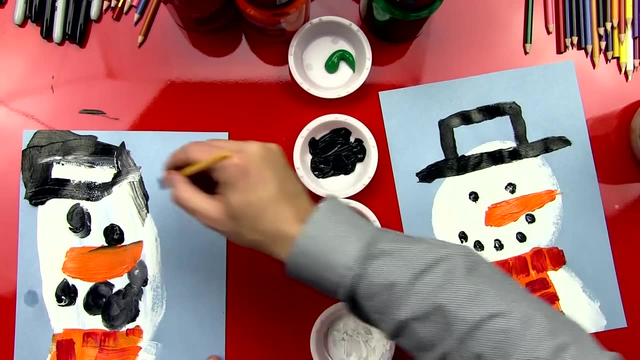 Yes, That's okay, You can do a lot, See that, And we do a big line across the bottom. Yes, And you can go see how I went a little further, A little off. Look at this right here, See this part. Yeah, You can do a little further right there. 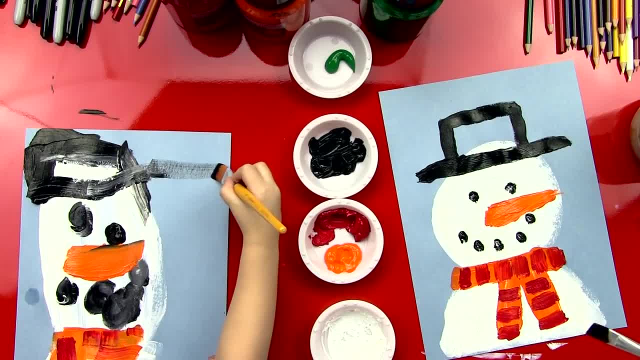 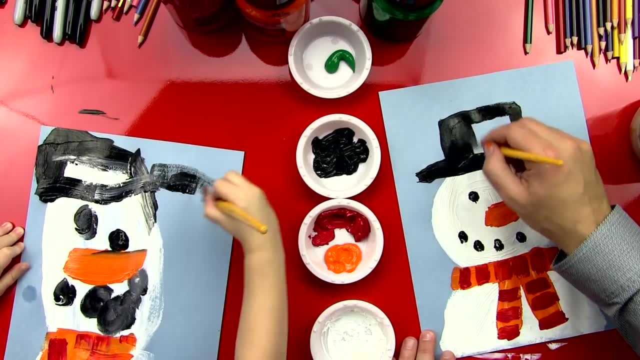 Yeah, You can go a little further out here. Good job, Do you need a little more? Yeah, And then we're going to paint it in. Okay, Like this: Paint your square in your box, your hat, I did. Oh good, You want to get it a little more black? 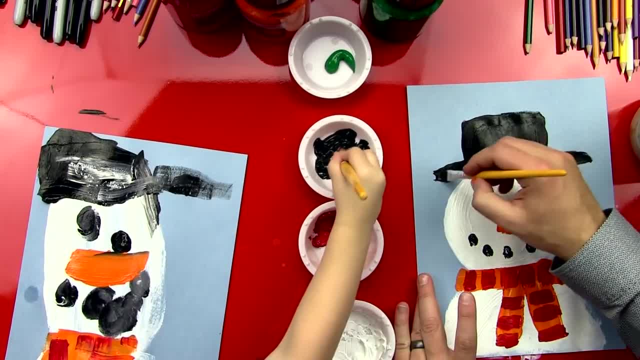 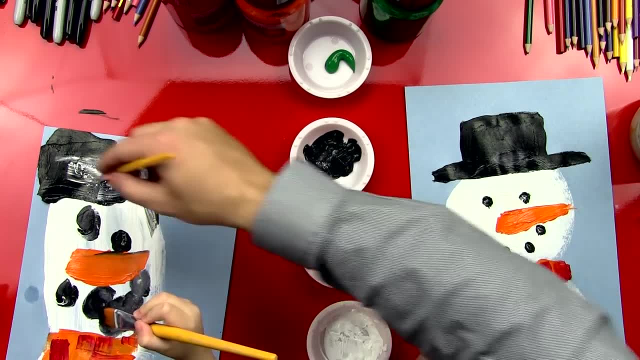 That's okay, It's kind of easy. It's kind of easy. I'm glad it's kind of easy. It's got a little bit white in it, Uh-huh. Okay, Cover up that white right there, so his hat looks. 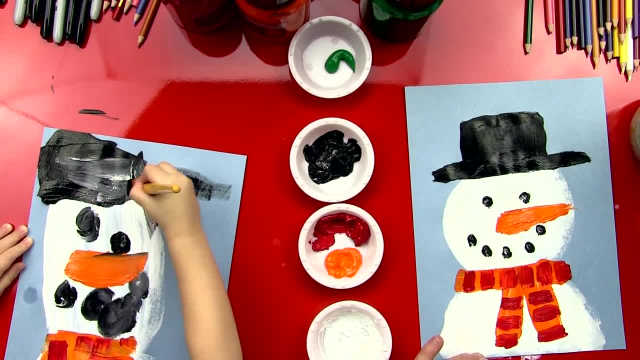 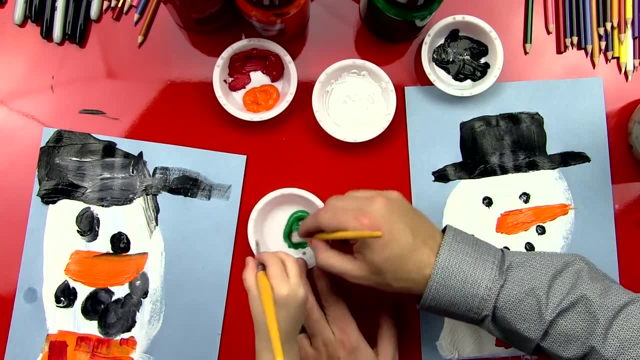 black. There you go, And then we're going to rinse off our paintbrushes. We're almost done, Okay, Yeah, All right. Okay, Now we're going to get some green. Can you get green on your paintbrush? 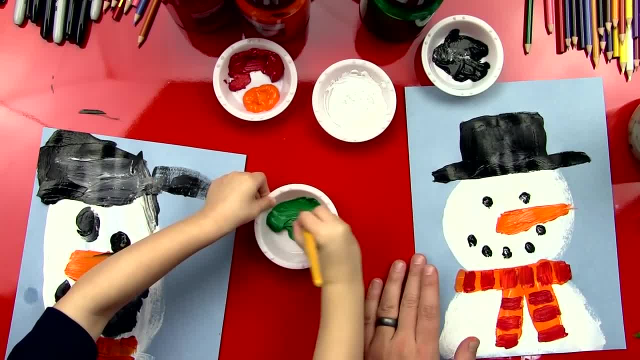 Yeah, And we're going to put some holly in his hat, Okay. Okay, So we're going to put a little leaf in there, Okay, And then we're going to put some holly in his hat, Okay, So we're going to put. 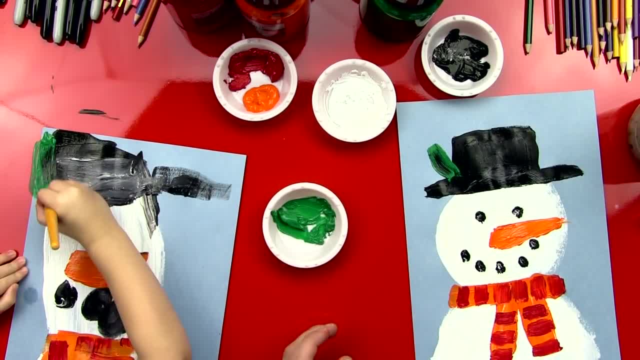 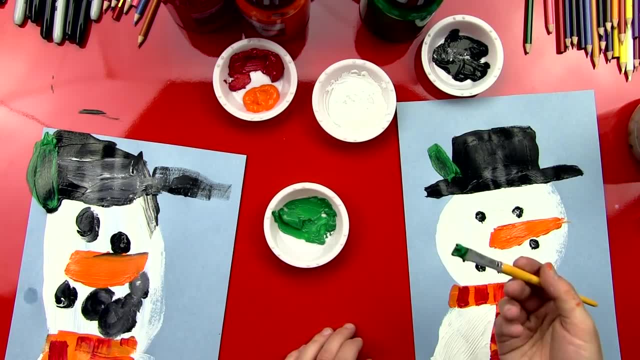 a little. leaf right here, Leaf right there, Yep, Oh, good job. You kind of ran out of room on that side. huh, Look, That's okay, We'll clean it up. It cleans up really easy And we're done with the. 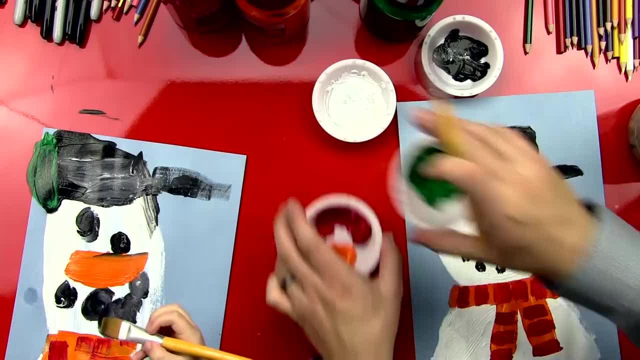 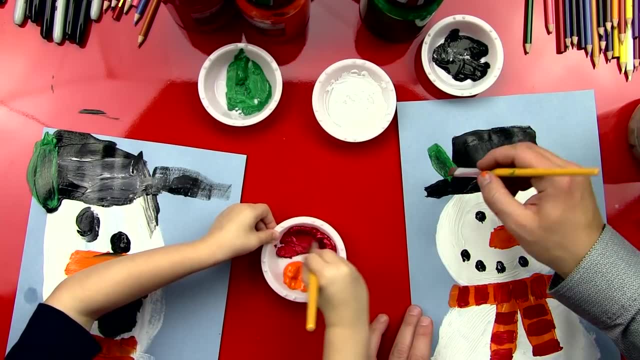 green. So we're going to get a little more red and we'll put the berries on. Okay, Now let's get some more red and we're going to do dots again. Okay, You ready? Yeah, Do one. Oops, I need a. 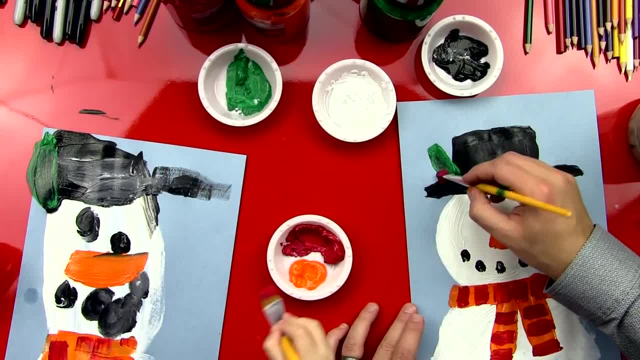 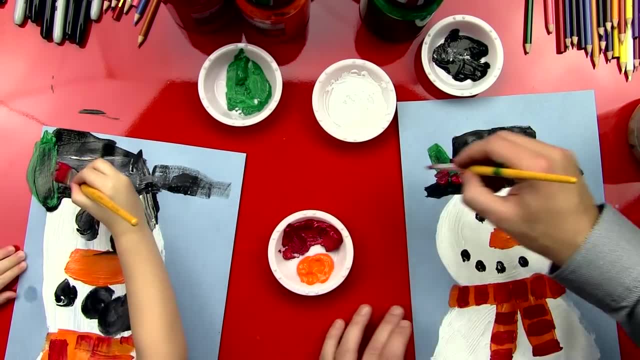 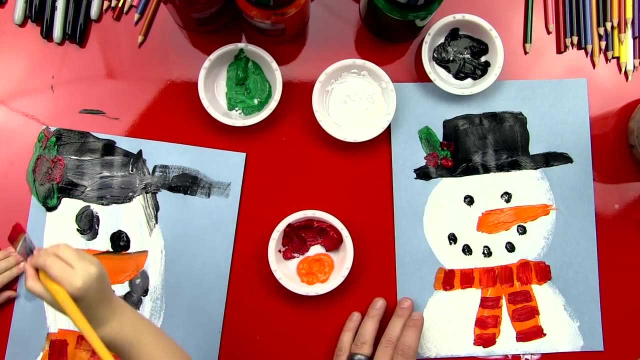 little more. I got a lot. Did you get a lot? One, Actually, I don't. Two, Three, Three dots. That part of your painting has a ton of paint. That's awesome. It's really thick over there. That may take a little while to dry. Yeah, That's okay, We're going to love it. 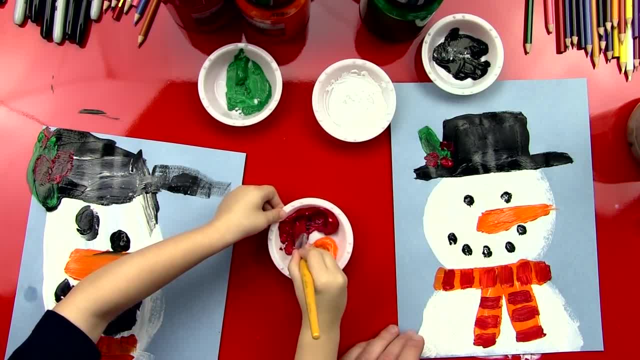 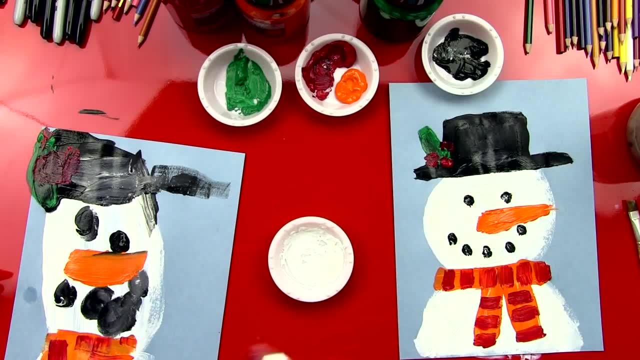 though I need a little more. You need a little more red for your berries, Yeah, Okay, Good job, That is one big berry over there, All right? Okay, So we're going to paint. We're going to rinse one more time. All right, We got a really teeny paintbrush for this one And we're going to 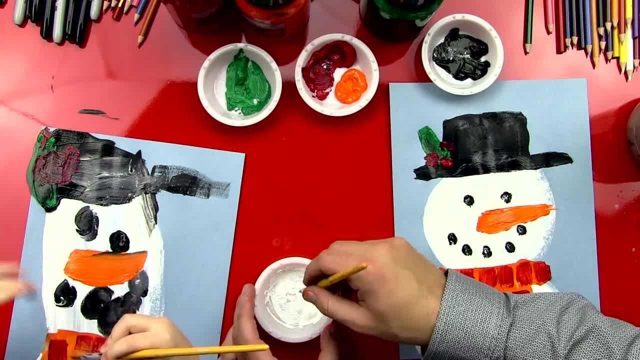 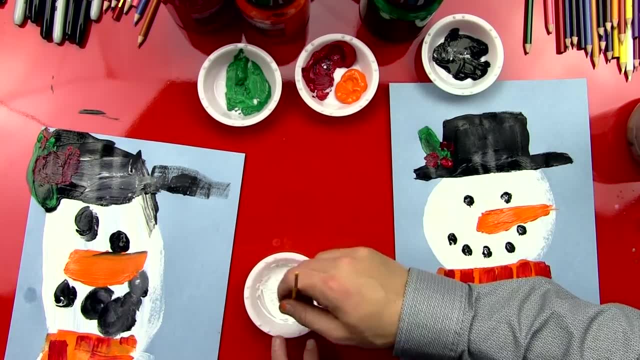 do our last step, And this is for Put water on it. It's okay, This is for the snowflakes. So we got little paintbrushes, We get a little bit of paint on there, Okay, Okay, And we do little.